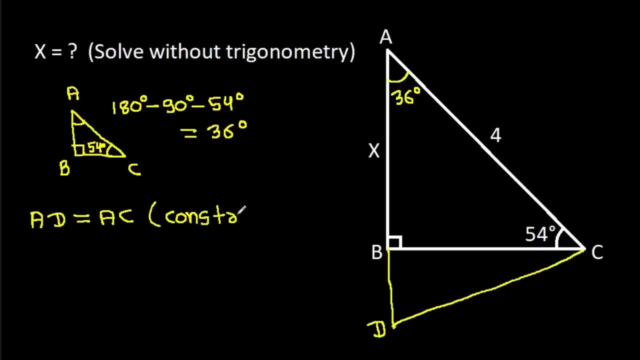 It is our correct angle construction. then in triangle ADC we have: AD is equal to AC and AC is 4, so AD it will be 4 and these two angles they will be equal. suppose theta and this angle it is 36 degree. 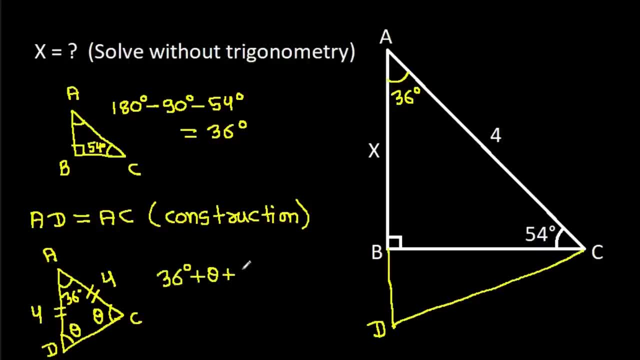 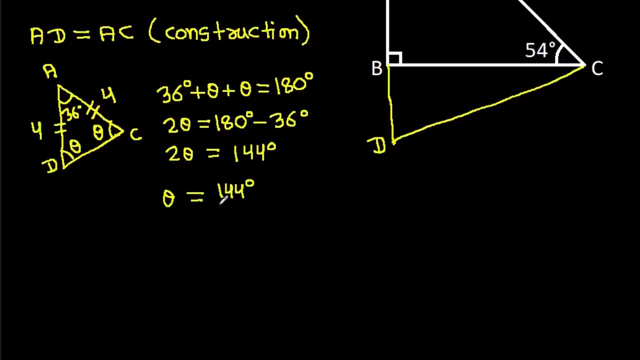 so 36 degree plus theta plus theta it will be 180 degree and 2 theta it will be 180 degree minus 36 degree and 2 theta. it is 144 degree and theta it will be 144 degree by 2, that will be 72 degree. 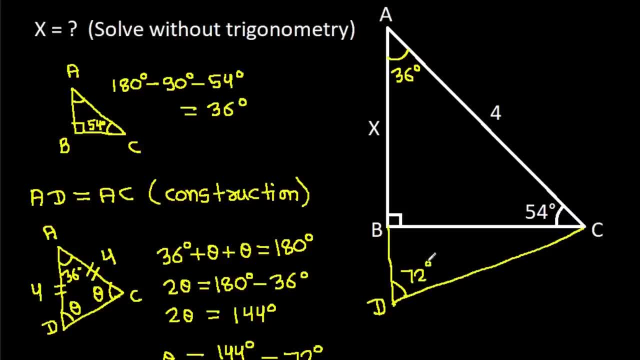 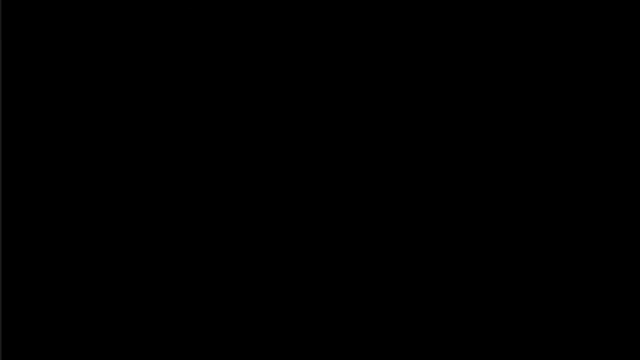 so this angle, it is 72 degree, and this angle, it will be 72 degree minus 54 degree, that will be 18 degree. it will be 18 degree and this angle, it will be 90 degree, and that will be a equal 1980 degree. 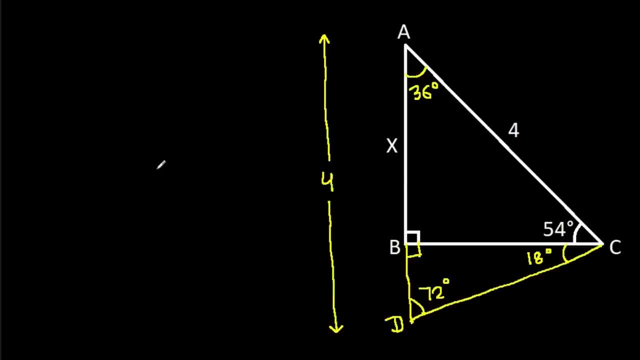 We have: AD is 4 and AD it is AB minus BD, and AD is 4. it is equal to: AB is x plus BD, so BD be 4 minus x, BD it is 4 minus x. and now suppose this point is E, such that BD it. 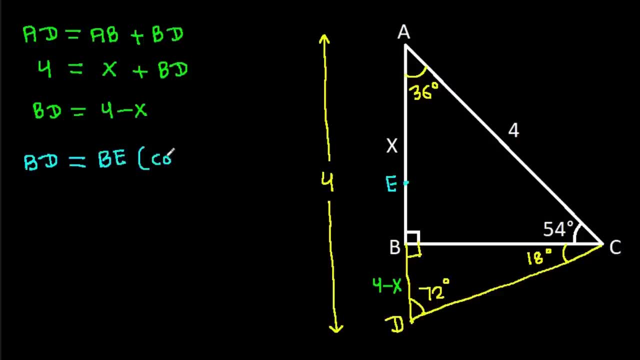 is equal to BE. it is our construction. and we have AB is x and BE it is equal to BD. so it will be 4 minus x And we have: AB is equal to x and AB is aE plus BE. that is x and it is aEE buckus. BE is 4 minus x. 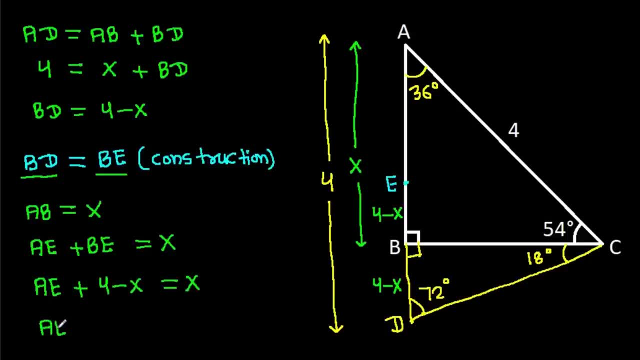 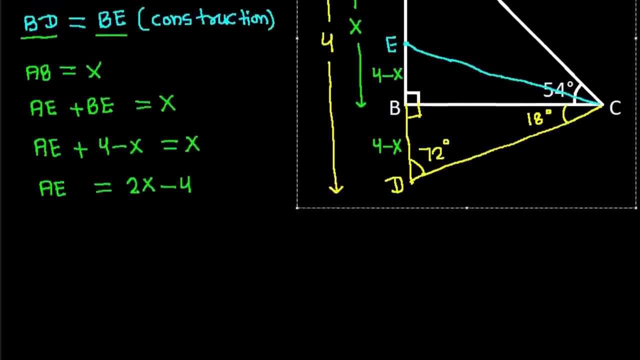 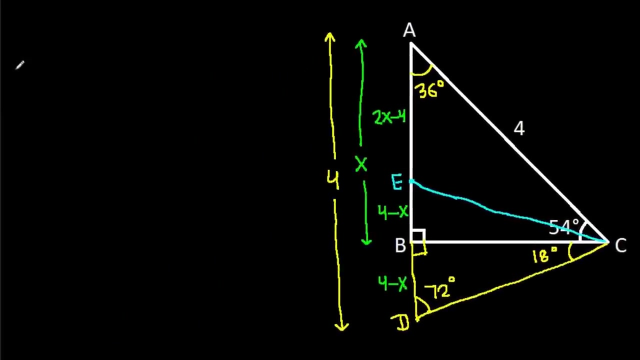 it is x. so AE it will be 2x minus 4.. it will be 2x-4. and if we join ce then in terangle cbd and terangle cbe cb is common angle, cbd it is equal to angle cbe, that is 90. 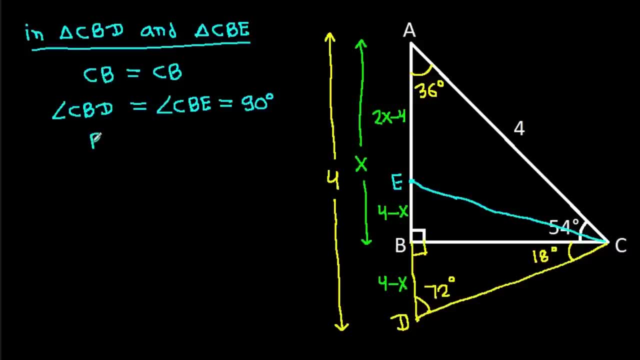 degree and bd it is equal to be, that is, 4 minus x. so terangle cbd it will be congruent to terangle cbe, hence angle CDB it will be equal to angle CEB. so this angle it will be also 72 degree and CD. 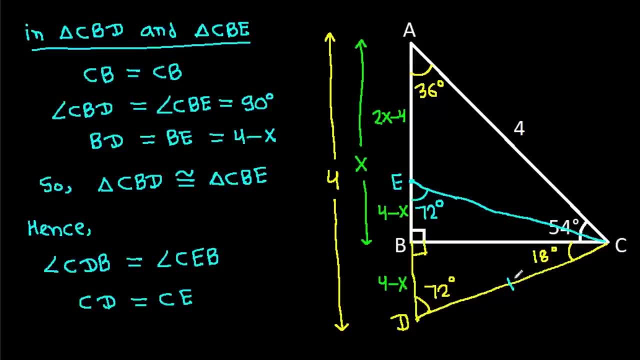 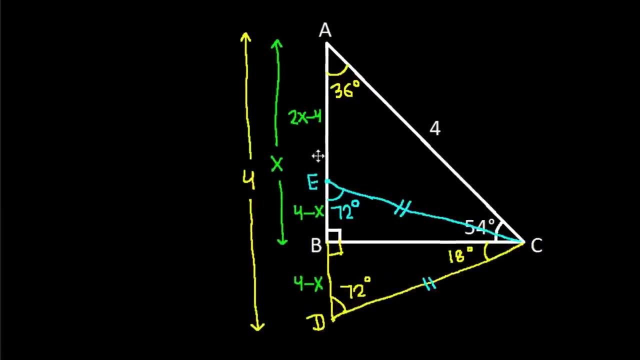 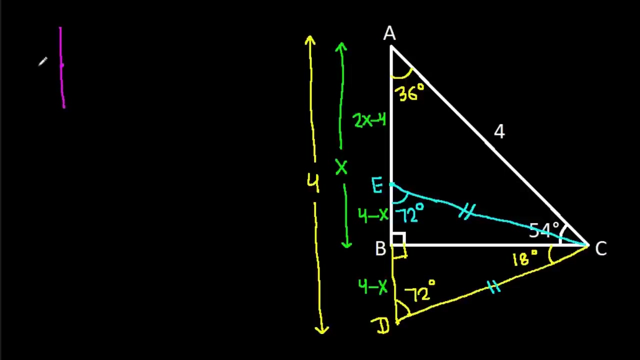 it will be equal to CE, CD, it will be equal to CE. and now, at point E, this angle is 72.. Now, at point E, this angle is 72.. Now, at point E, this angle is 72.. So this angle, it will be 180 degree minus. 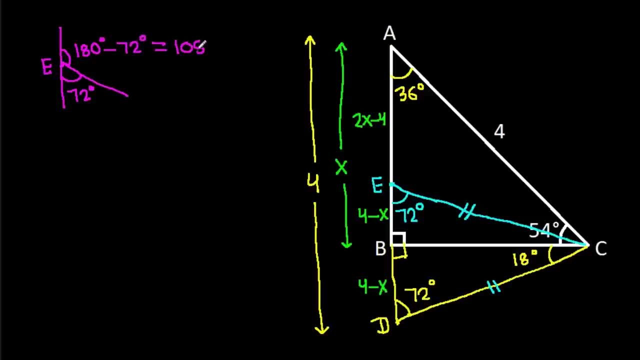 72 degree, that will be 108 degree. This angle, it will be 108 degree. And now, in triangle A, E, C, this angle is 108 degree, This angle is 36 degree. So this angle, it will be 180 degree minus 108 degree minus 36 degree. 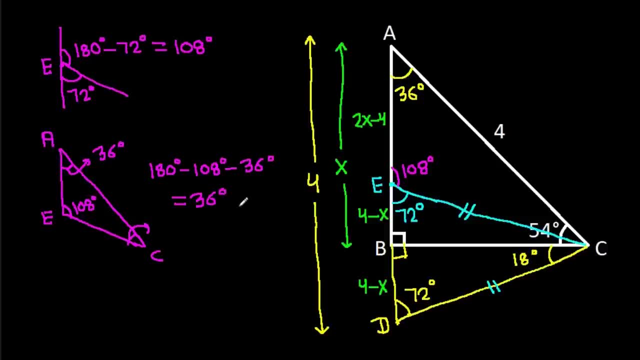 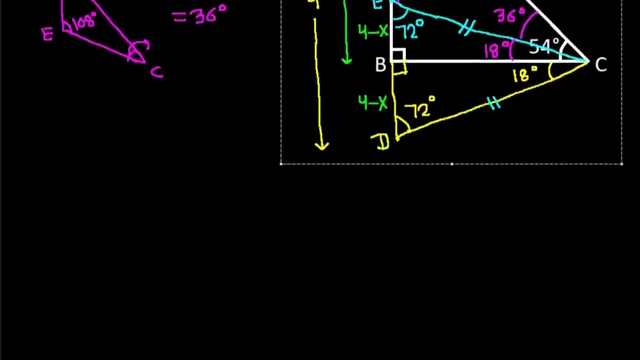 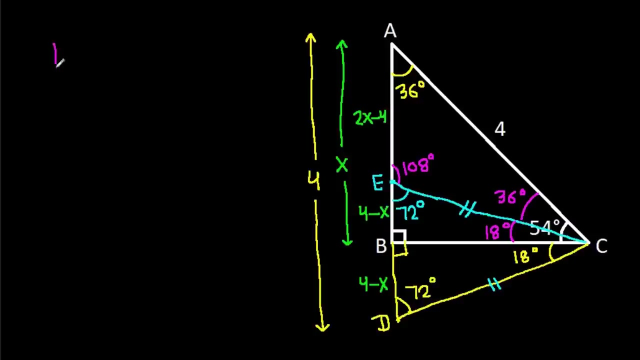 That will be 36 degree. So this angle, it will be 36 degree, and this angle, it will be 54 minus 36.. That will be 18 degree. And now in terangle AEC, these two angles are equal, that is 36. 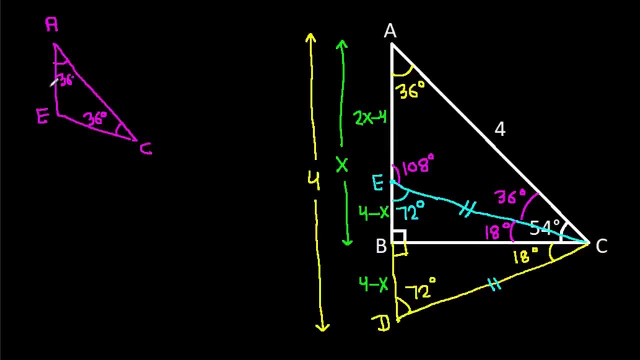 degree, So Ae it will be equal to Ce, and Ae is 2x-4,, so Ce it will be 2x-4, Ae- it is equal to Ce- that will be 2x-4. and Cd is equal to Ce, so it will be also 2x-4. 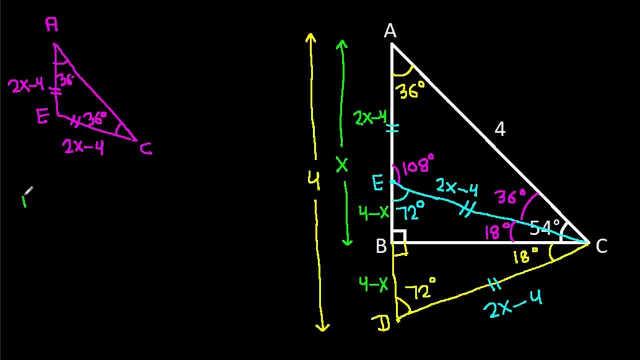 And now in terangle Adc and terangle Cd it will be 2x-4.. We have: angle Adc is equal to angle Cde, that is, 72 degree, and angle Acd it is equal to angle Ced, that is 72 degree. 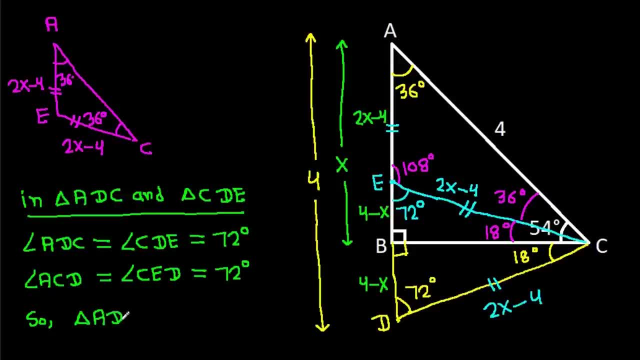 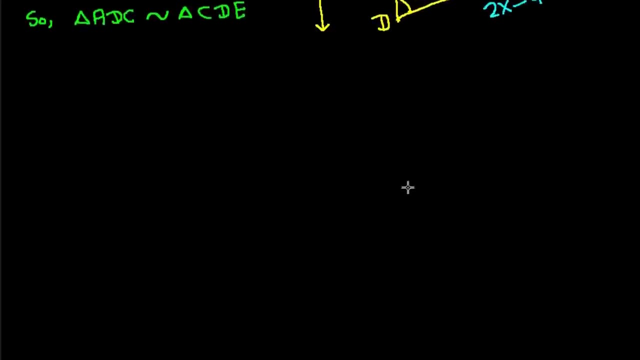 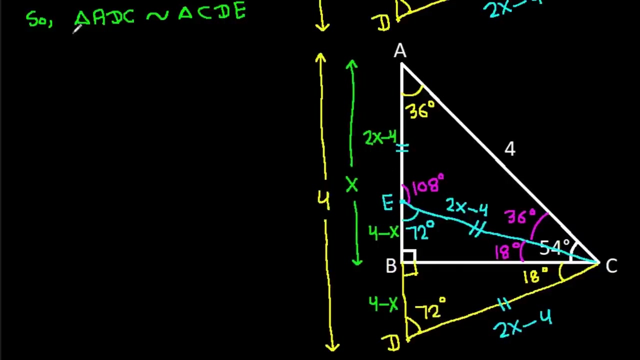 So terangle Adc. it will be similar to terangle Cde and these two terangles are similar, Hence Ac by dc, it will be equal to Ce by De, and Ac is 4 by dc is 2x-4, it will be equal to. 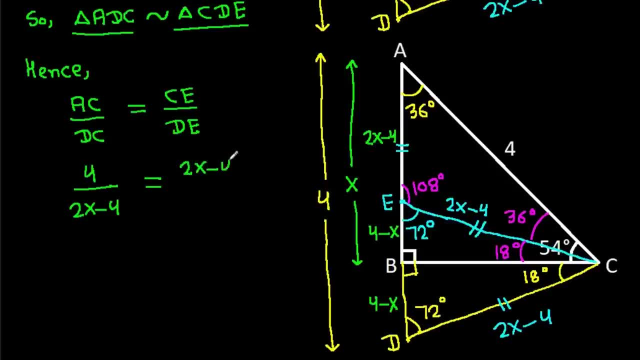 Ce is 2x-4 by De, So it is 4 minus x plus 4 minus x. that will be 2 times 4 minus x, and if we cross multiply, then 4 times 2 times 4 minus x, it will be equal to 2x minus 4 times 2x minus 4and it. 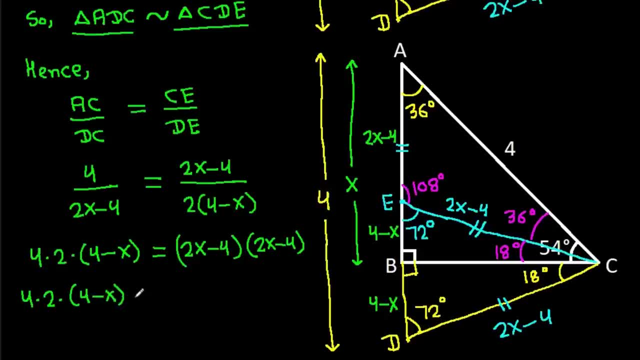 It is 4 times 2 times 4 minus x is equal to 2x minus 4, it is 2 times x minus 2 and 2x minus 4, it is 2 times x minus 2 and 2 times 2, and 4 will get cancelled. 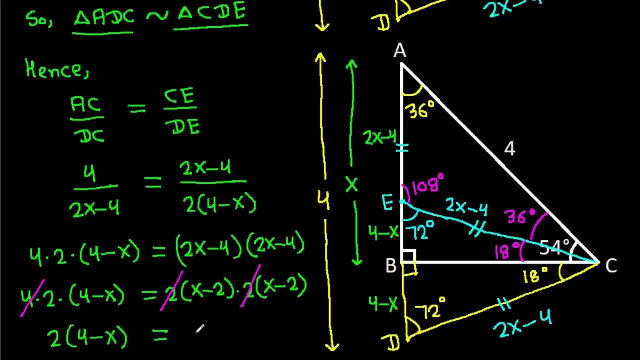 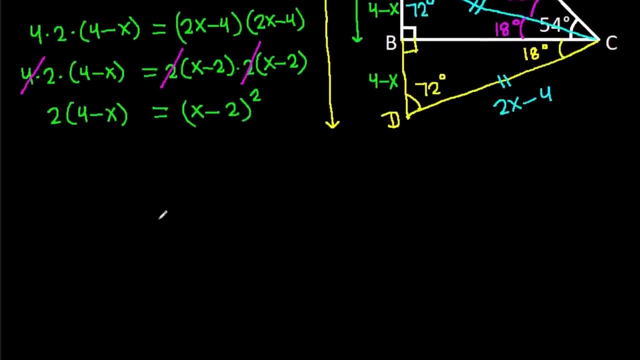 So it is 2 times 4 minus x, is x minus 2 a squared, and it is 8 minus 2x. is equal to x square plus 4 minus 4x, And it is x a squared and minus 4x minus 2x. 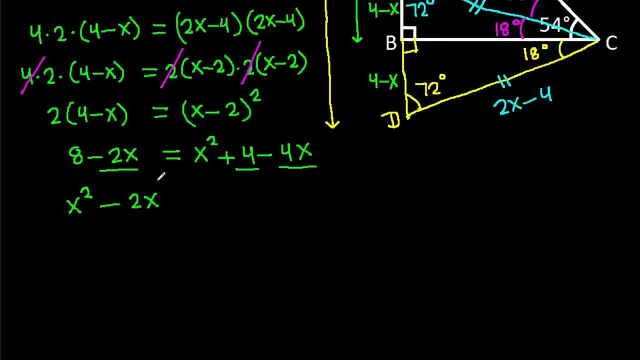 4 minus x will be minus 2x, and 4 minus 8, it will be minus 4, that is 0.. And for equation axs square minus bx minus c is equal to 0, x is minus b minus minus a square root of b square minus. 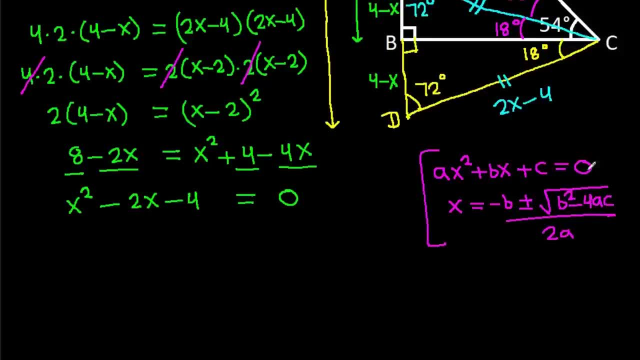 4ac by 2a, And here a is 1, b is minus 2, and c is minus 4.. So x, it will be minus b of minus 2 plus minus s square root of minus 2 s square minus 4 times 1 times minus 4 by 2 times 1. 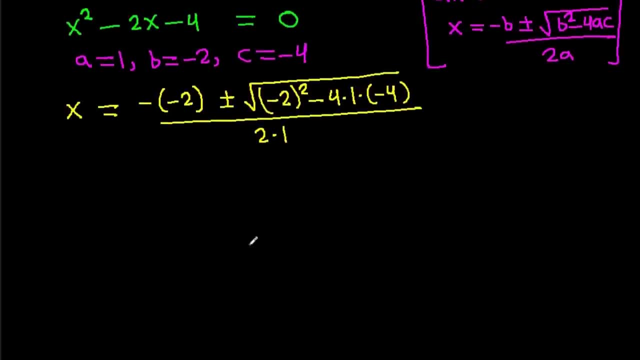 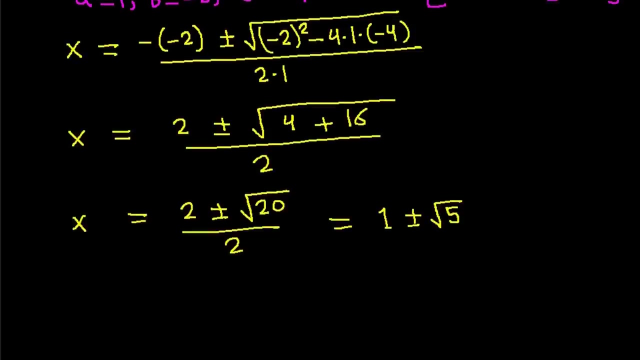 and x is equal to 2 plus minus s square root of 4 plus 16 by 2, and x is equal to 2 plus minus s square root of 20 by 2, and if we divide by 2, then it will be 1 plus minus s square root of 5.. So we get: x is 1 plus s square root of 5 and x is 1.